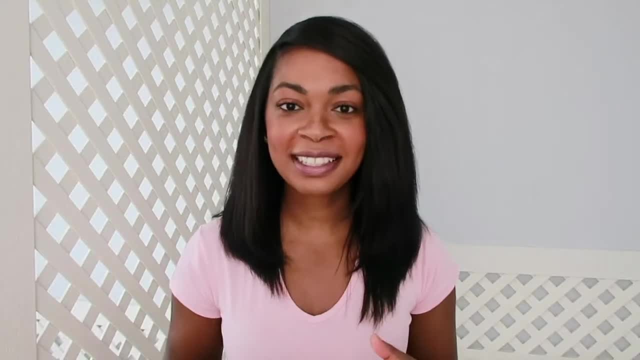 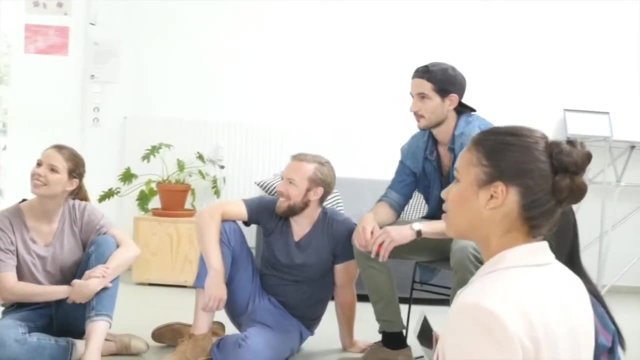 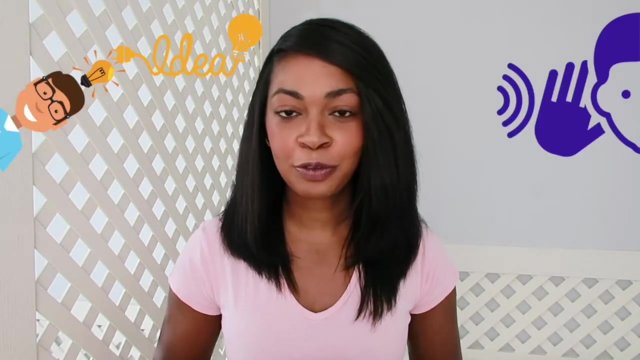 a circle with four to ten people. one person gets up for about 20 seconds to continue a story. after your 20 seconds are up, you sit down and you let the next person continue telling that story. the goal of this game is for you to develop your listening skills and for you to use your 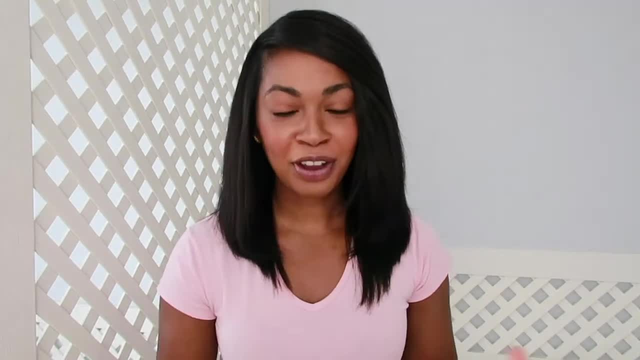 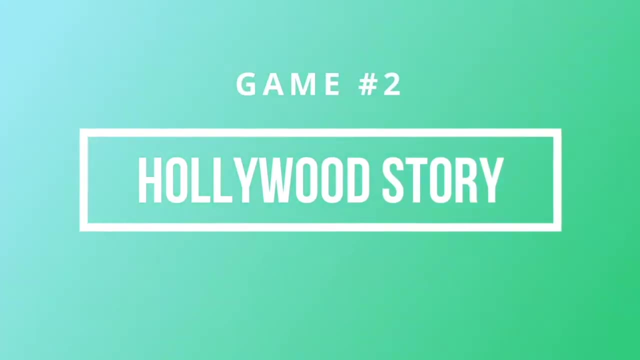 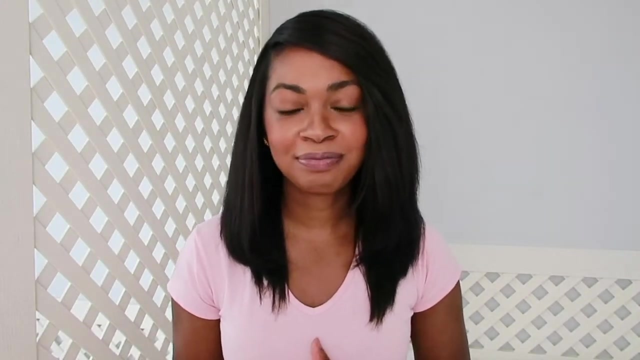 creativity to develop stories. remember if you're the next person speaking. that story needs to continue making sense as it unfolds. game number two is called the hollywood story. the hollywood story game can be played in a small group or on your own, just in front of a mirror. 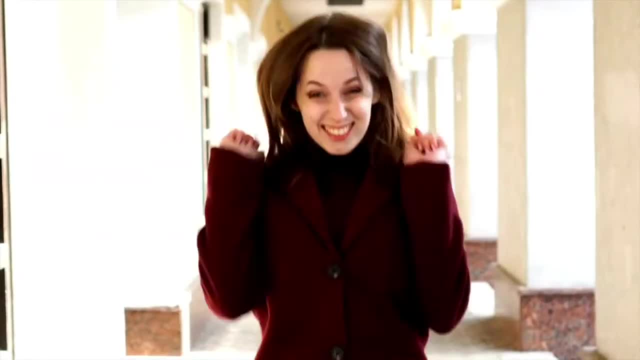 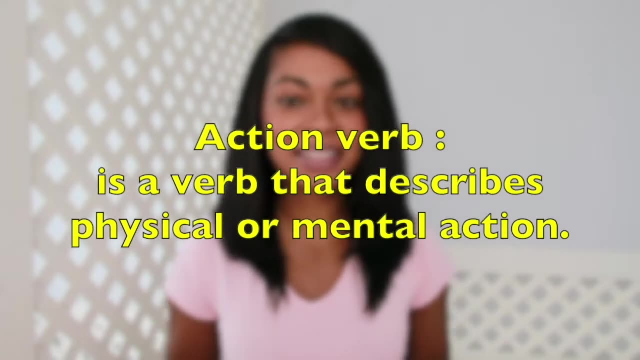 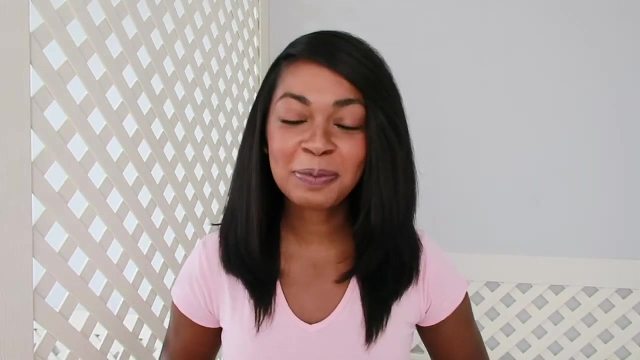 in this game, you need to tell a story using as many action verbs as you can think of. an action verb is a type of verb that describes physical or mental actions. in other words, you need to express physical or mental actions in this fun public speaking game for every action verb that you use. 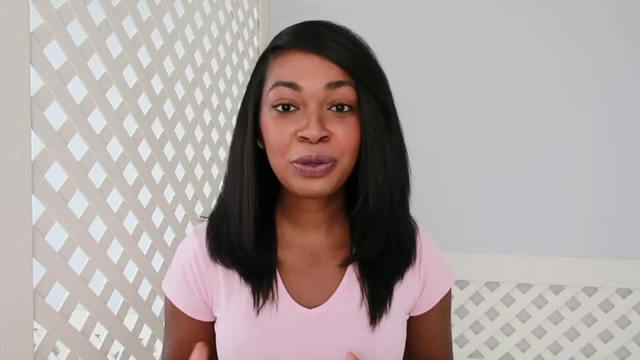 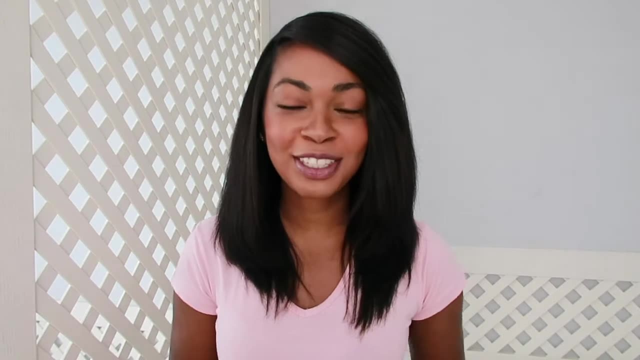 in your story. you need to act up that word using your body language and your gestures. here you're trying to mimic or match the action verb with your body language and your gestures. you're trying to mimic or match the action verb that you're using to your body language. 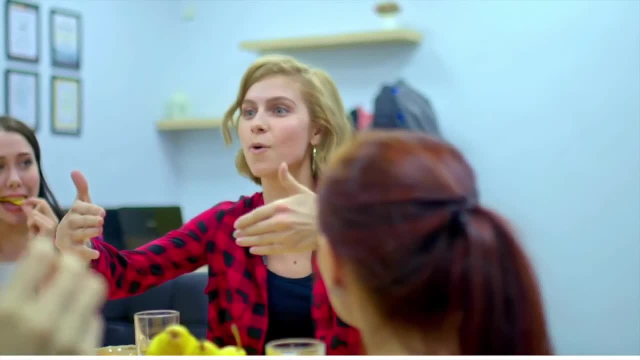 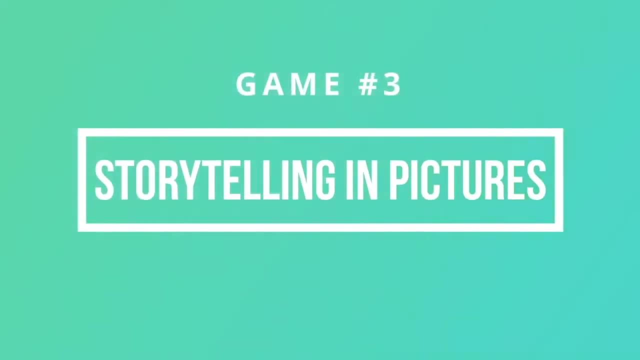 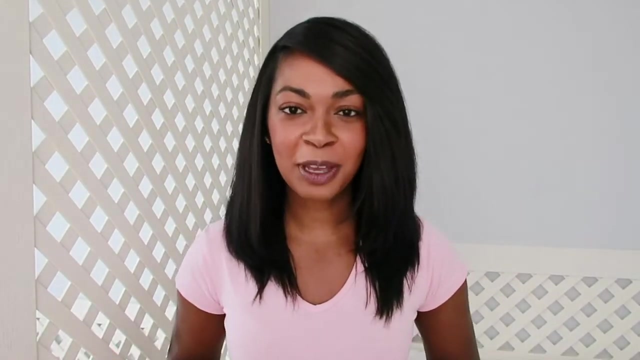 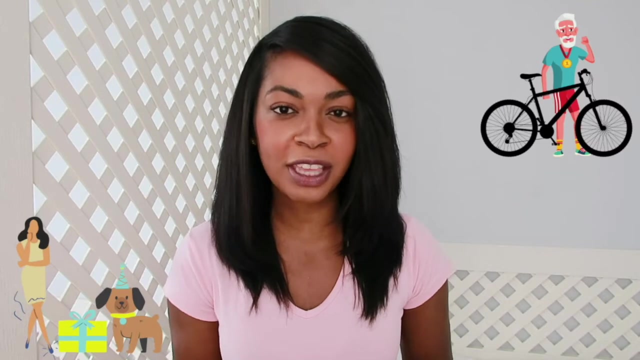 oh, and, by the way, speaking with your voice and your body language actually makes your speaking more compelling. game number three is called storytelling in pictures. this game, right here, is my all-time favorite game when it comes to storytelling and pictures. you need to put about five photos in a folder. you can use animals, events, people, sporting equipment- you name it. 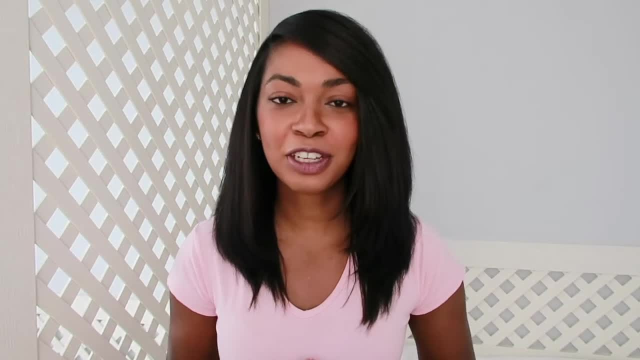 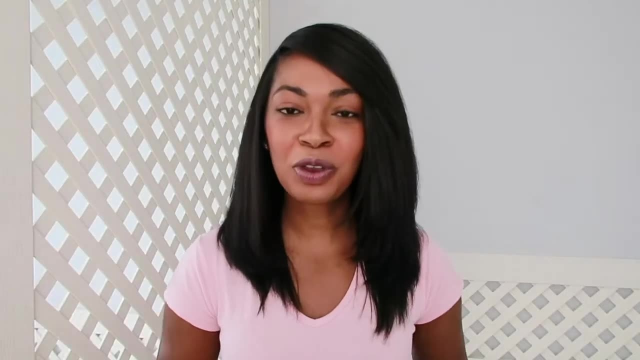 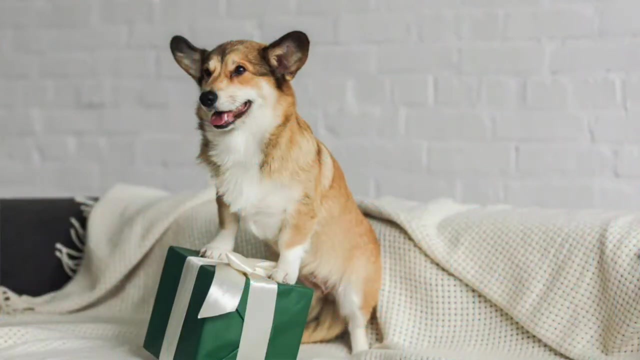 in order for things not to get way too complicated, you need to make sure those photos look as simple as possible. it could be an image of a volleyball, for example. after you've put all your five images in one folder, turn on your big screen or your full view and click through. 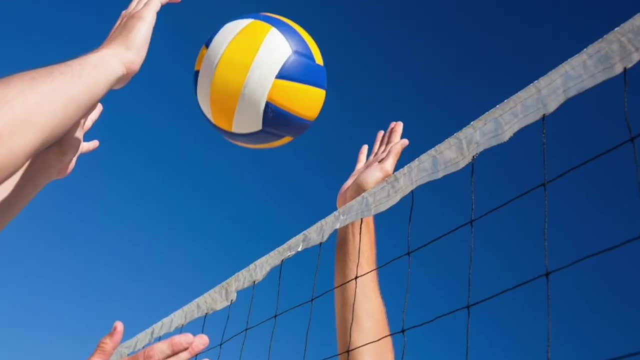 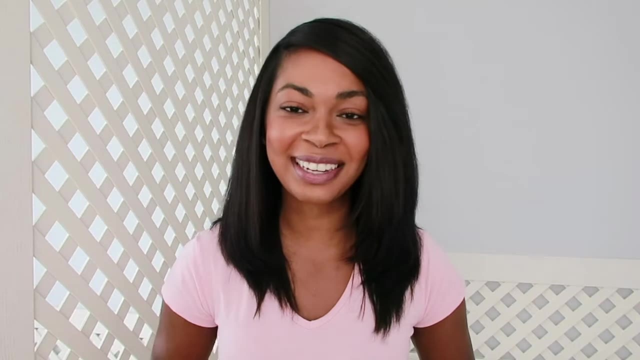 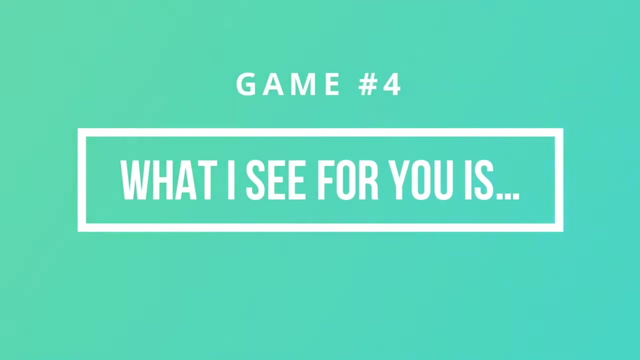 one image at a time. as you click through each photo, the speaker will share a story using one to three sentences related to the image that shows up on the screen. speaking game number four, which also happens to be my last one, is called. what i see for you is this: 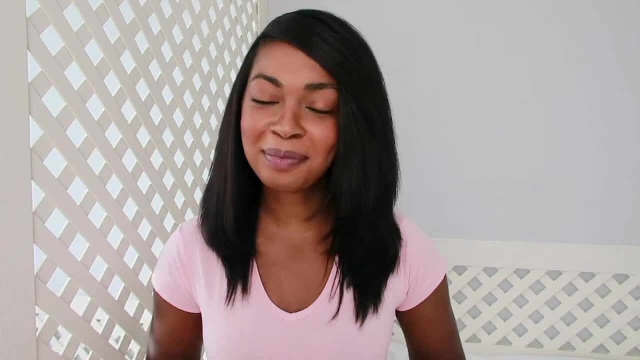 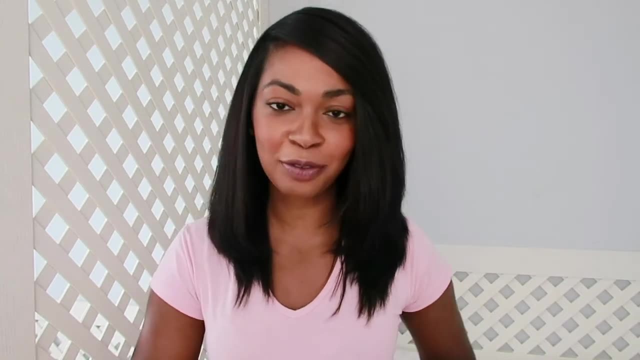 game can be played in smaller groups, in bigger groups or by yourself. all you do is stand up in front of the room, pick a friend that's also in the room and then you introduce that friend. however, instead of introducing that friend using the normal way, because everyone in the room already-